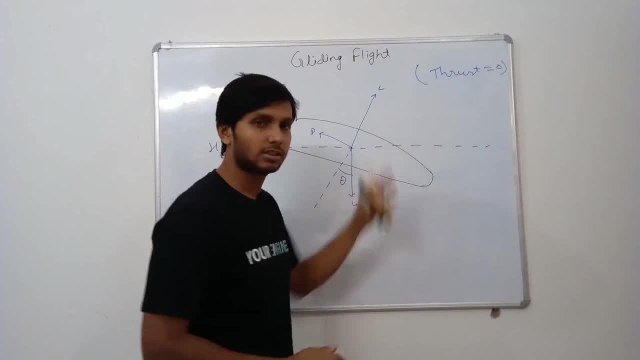 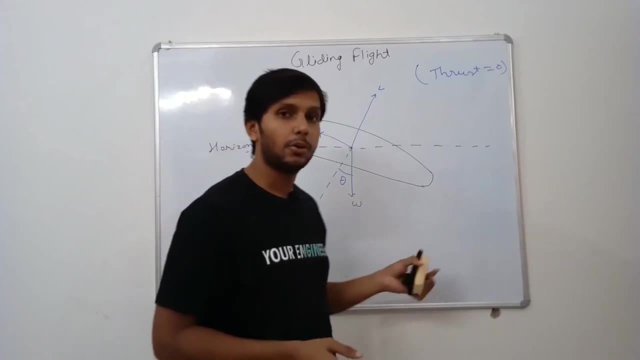 glide. there is no requirement of power at that time. okay, thrust is zero, we turn off our engine and we glide. so if we go to the numerical concept that we have to take out how much angle requirement will be that we glide, second, if we have to take out this, 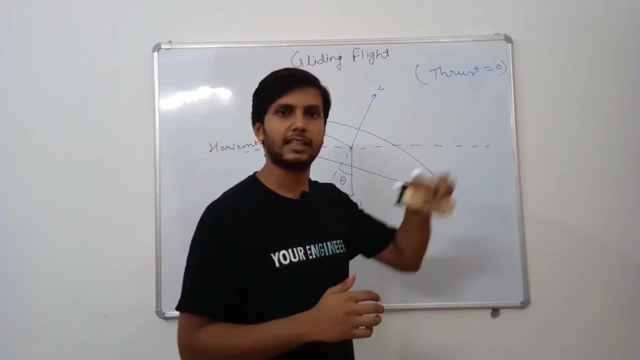 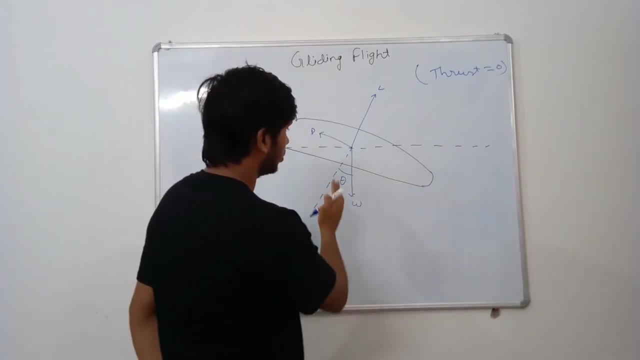 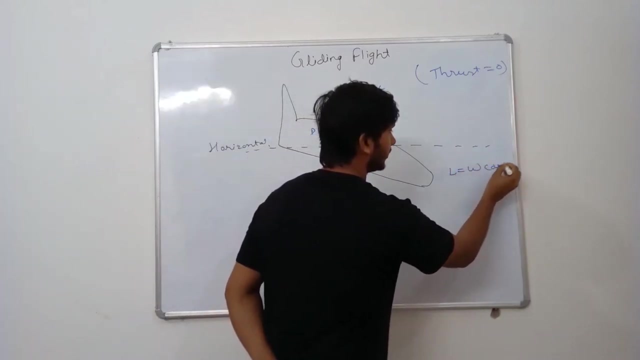 motion. whatever kind of range is there? how much range will it cover? at what particular aircraft? what height have you started glide? then lets hack into one thing: if we, which have seen the concept of vector, so w cos theta is equal to L, so L is equal to W cos theta and sin theta. component of w is the. 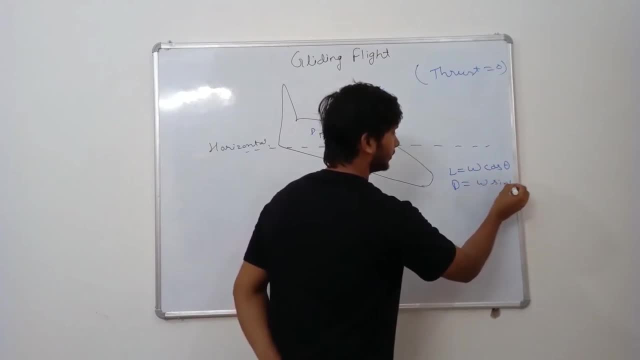 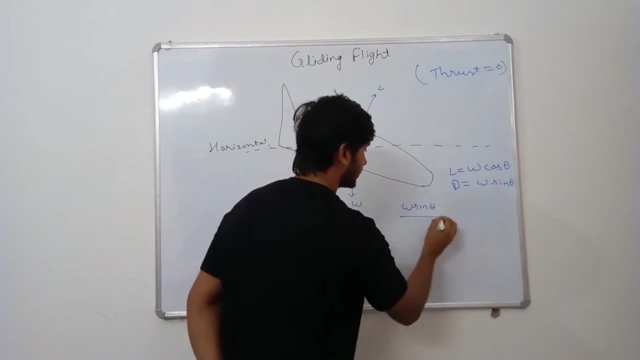 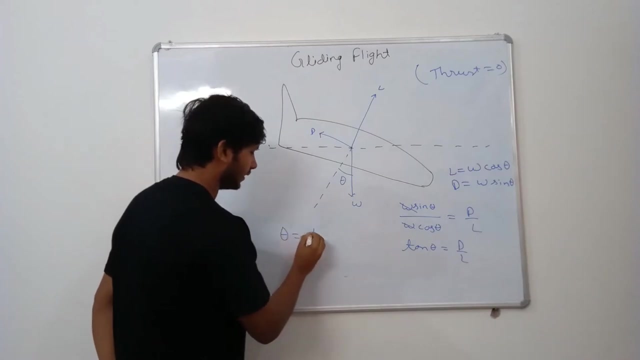 component of d, so d equal to W sin theta. okay, when we are considering here. so we sin theta upon W, cos theta is equal to D by L, W and W are cancelled. We got that tan theta equal to D upon L, which means theta equal to tan inverse 1 upon L by D. Now what? 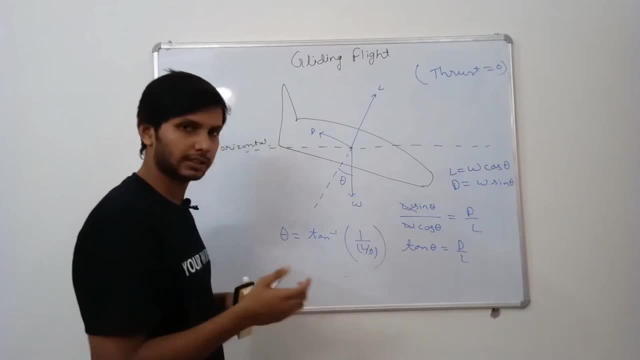 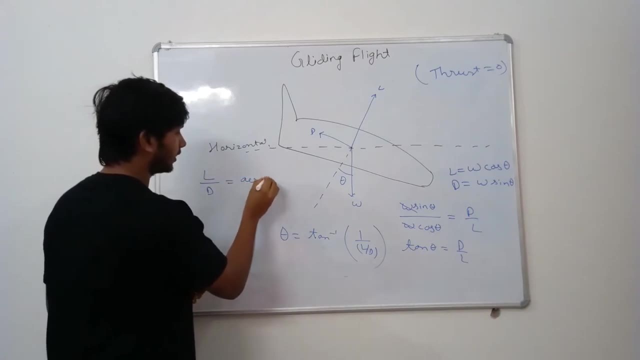 is L by D. L by D is aerodynamic property, which is also called aerodynamic efficiency. So L by D is aerodynamic efficiency, which depends clearly on the aircraft design. What are the design parameters? how much design lift coefficient we have taken? that will be. 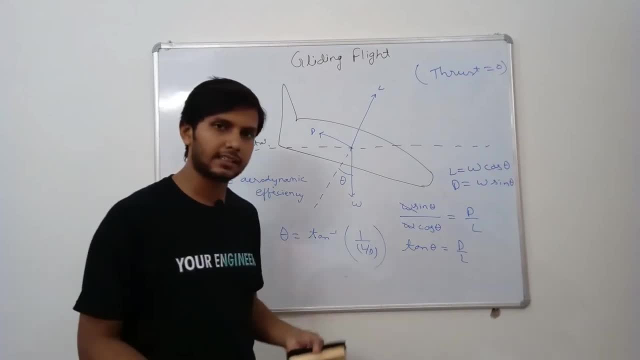 related that how much lift we will get, how much surfaces are there and what are the properties of surfaces. what is the paint? how much structure is taken, what are the viscous flow parameters we have taken? So all the design parameters are taken. 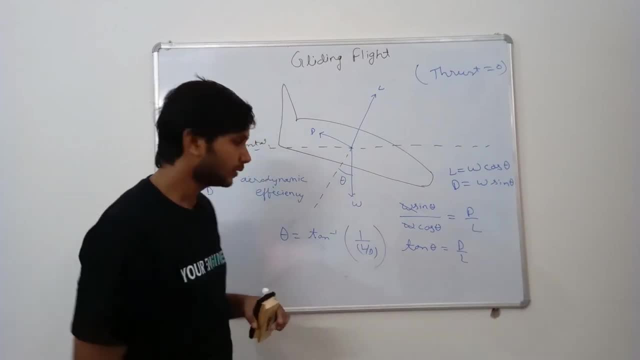 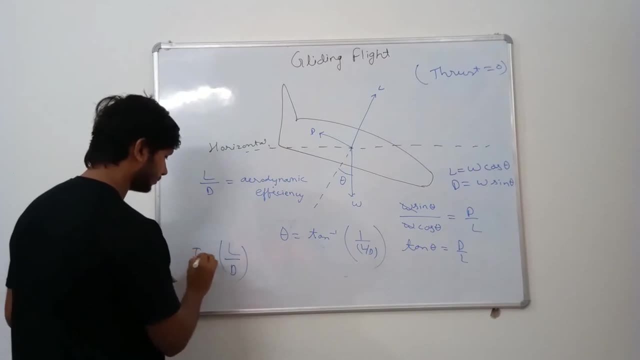 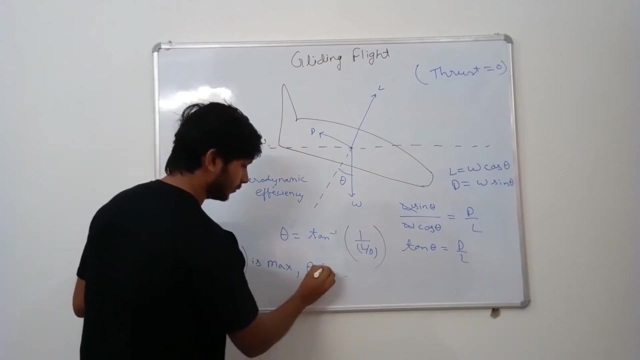 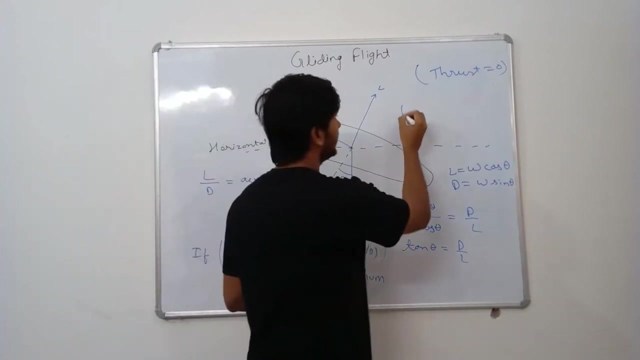 So L by D is aerodynamic efficiency, which depends clearly on the aircraft design. What are the design parameters of flat verschel energy? Well, my position is 0.. What is difference between difference among slbs? Nothing, Slipler Sliper. 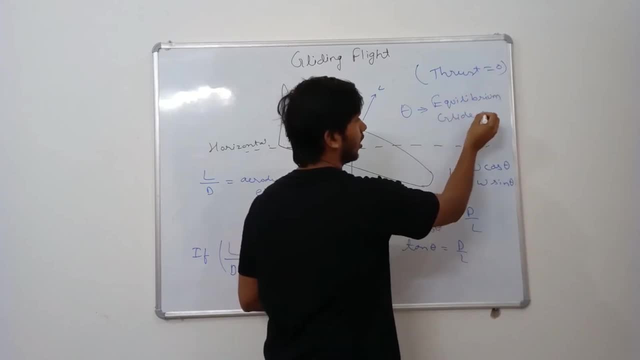 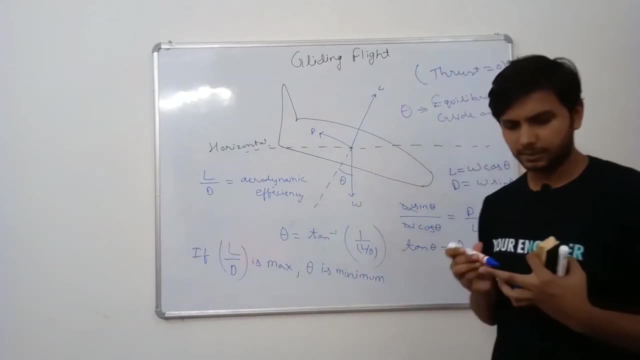 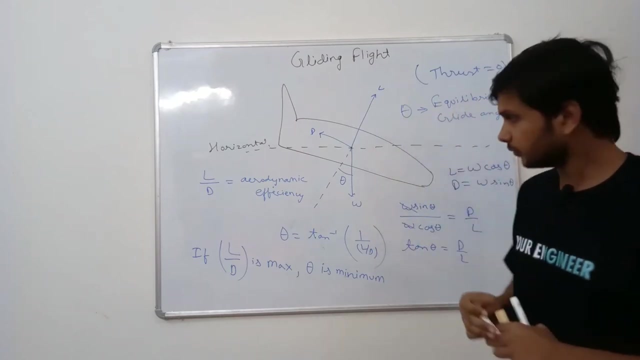 What? okay, if you prepare for gate exam, then also this theta is very much asked, okay, or it can be required in some particular way. maybe the question is somewhat twisted and you can be asked for theta, so this is the case, okay, if i want to make this question very tricky, then i will first give you. 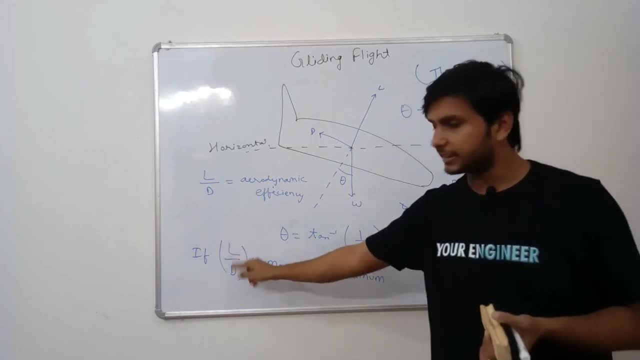 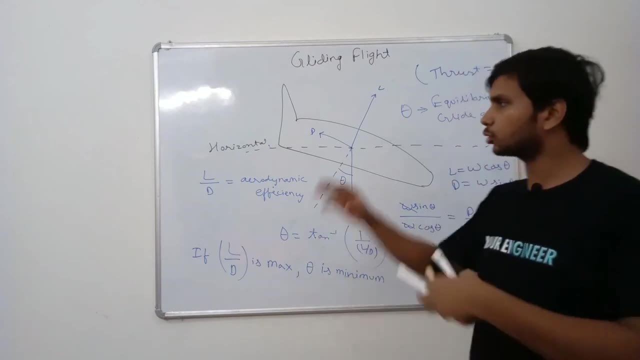 theta. okay, after giving theta, i will give you the relation between c l, c d, that is, c d equal to c d naught, plus c l, square upon pi ar. okay, with this question, i will try to get you some questions so we can twist the questions on the basis of glide angle. now, if we want to see this thing, 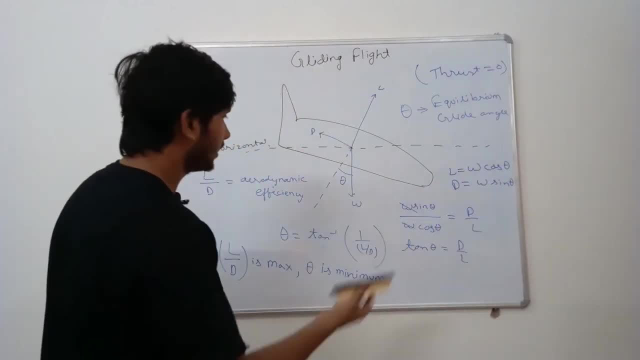 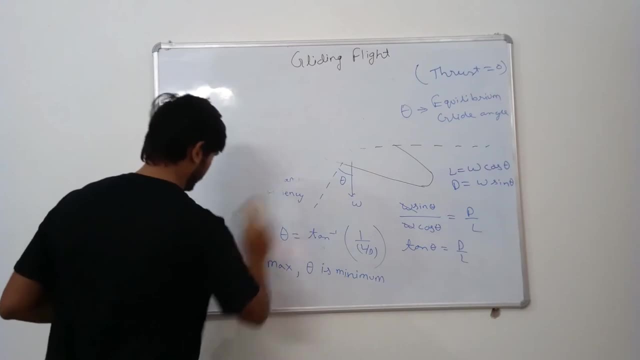 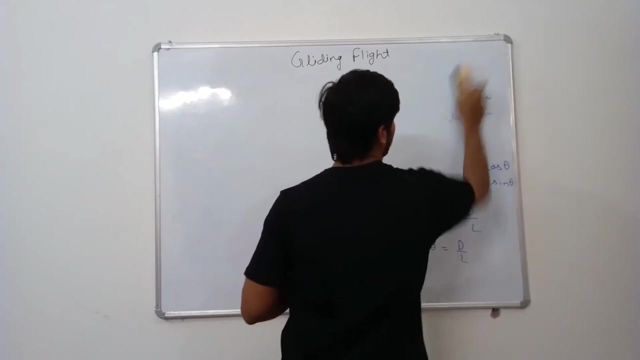 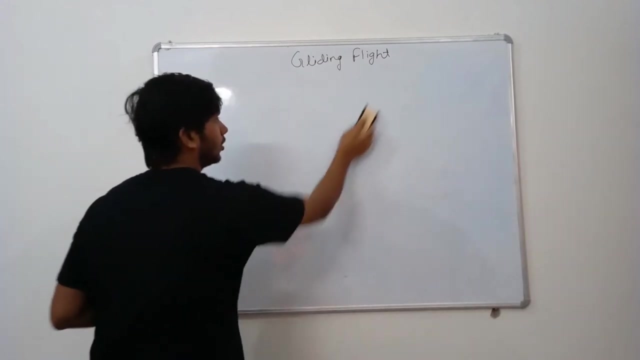 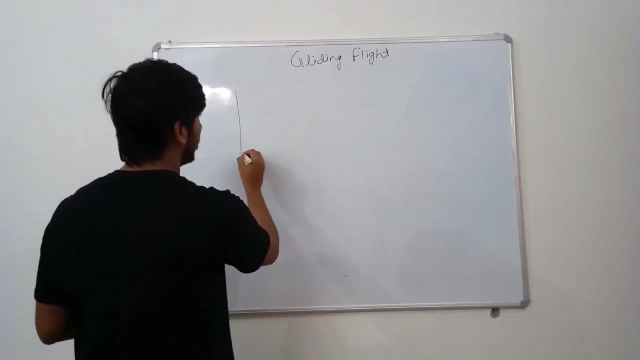 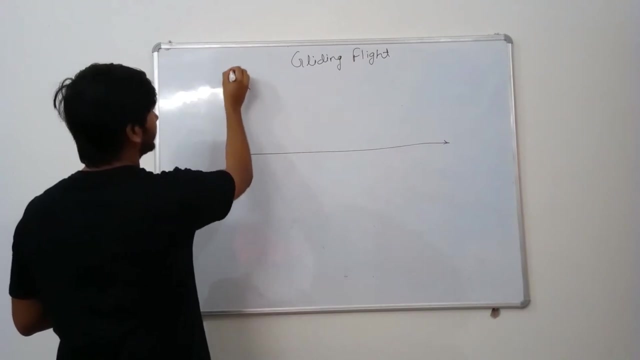 that. what will be the range of any particular aircraft? okay, while gliding. so let's see that too. so let's assume that. suppose that this is a particular height and this is a particular distance, and there is an aircraft which is gliding here. okay, we have taken an aircraft whose angle we had just told that it is theta. 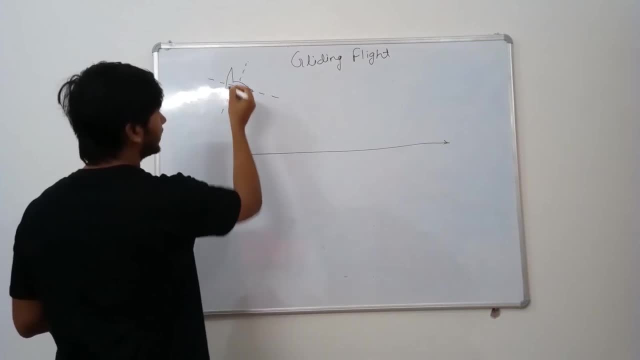 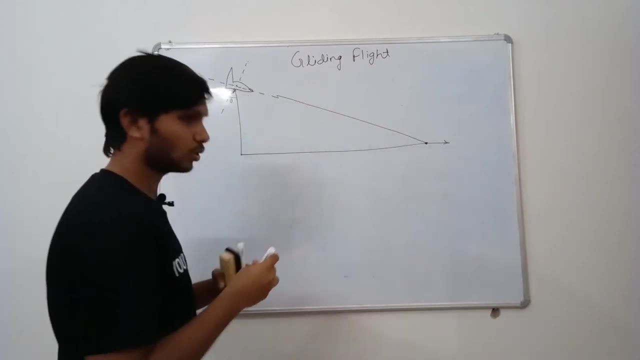 okay, so this is theta angle, and if it is gliding at theta angle, then it is theta angle. and if it is covering every aspect, then what will happen? suppose the aircraft moving forward is covering here till the distance. so here simple method of technometric is applied. 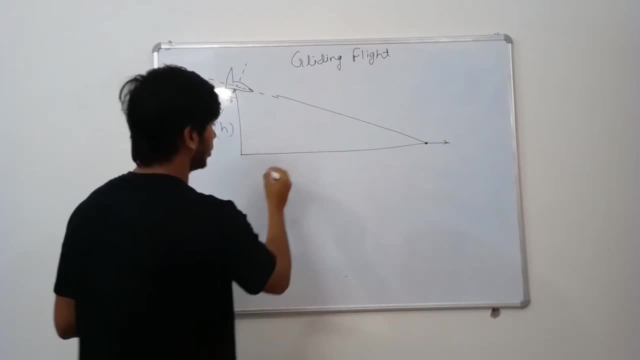 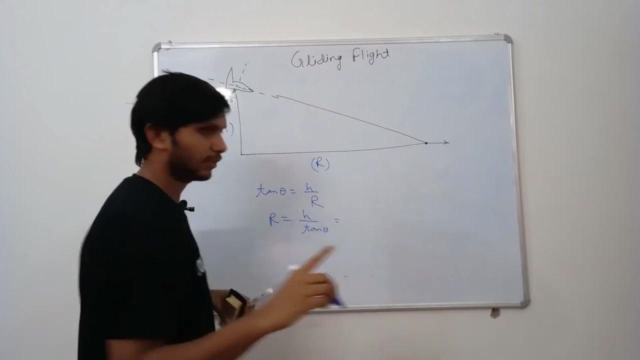 and this is if consider that this height is called h and distance is known as r. okay, so what will happen here? what will we change? the thing that if we want to take tan theta right, so tan theta will be h upon r, r h to H upon tan theta. We have already read the value of tan theta. What is it? d by L. 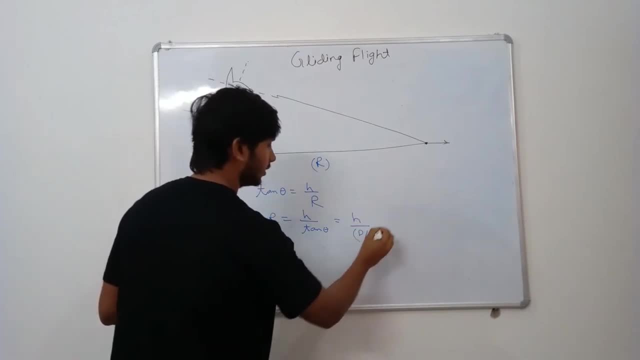 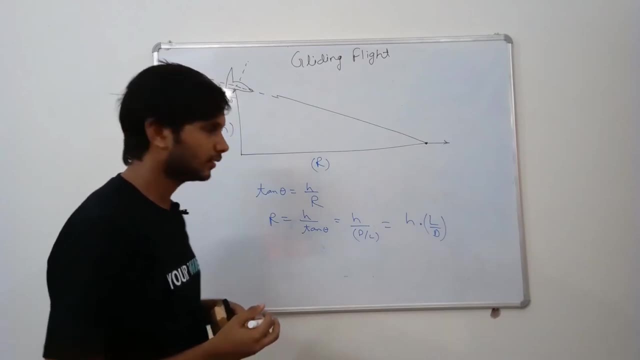 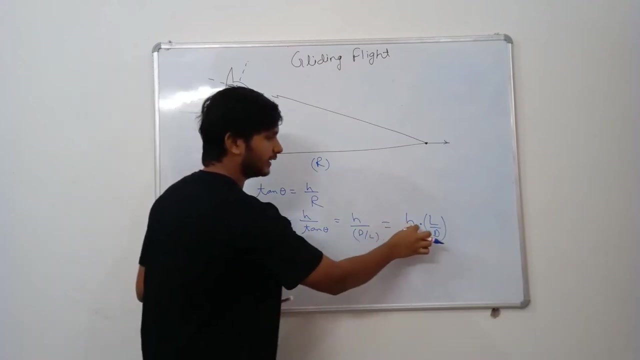 So H by d by L, which will become H into L by d. So this formula is given to you. This thing comes in gliding flight Range equal to height into L by d, L by d. we already know what is it: Aerodynamic efficiency. So the higher the aerodynamic efficiency, 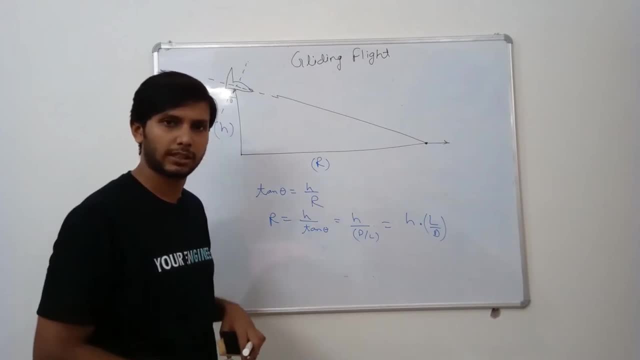 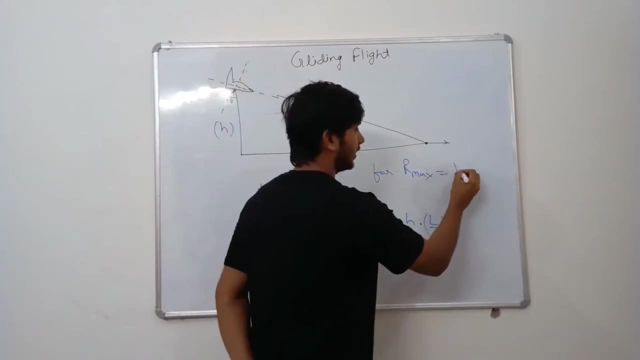 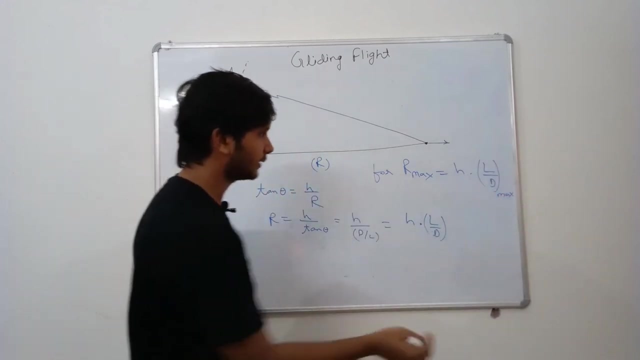 will be, the higher the range will be and the less angle requirement will be. So for R max you must need H into L by d max. If the ratio of lift and drag is maximum, then in that case the range will be maximum. How much runway length do we need? There is one. 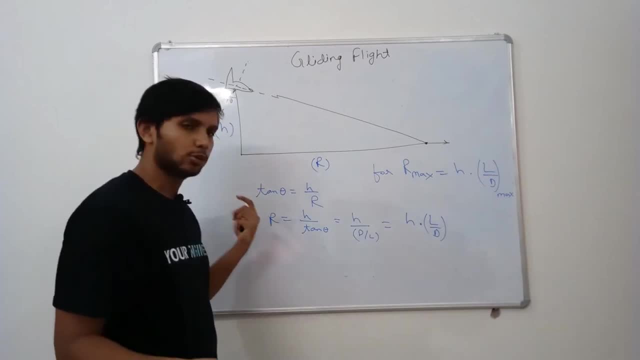 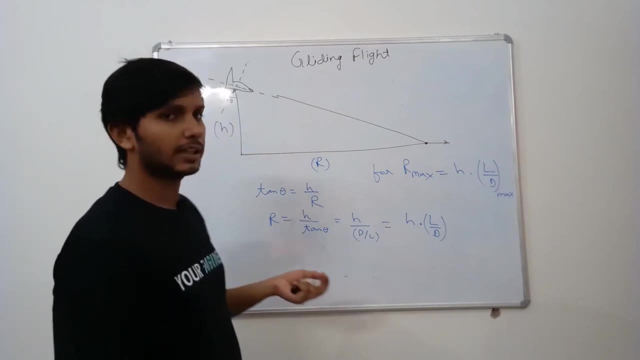 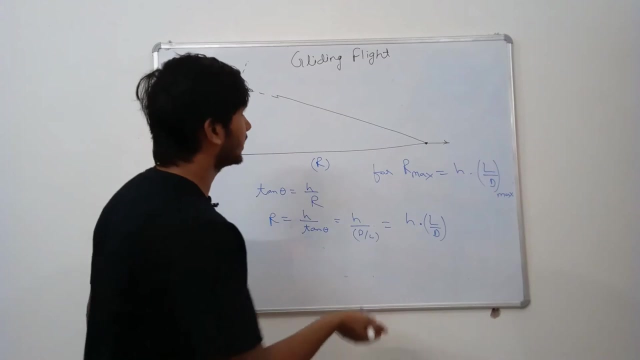 more concept. You guys note this thing, You guys see things. There is one more concept: that if we take the risk of velocity, Let us take the risk of velocity. in that respect, How much velocity requirement is there When the velocity will be more or less? What do we consider as weight? So if we see in 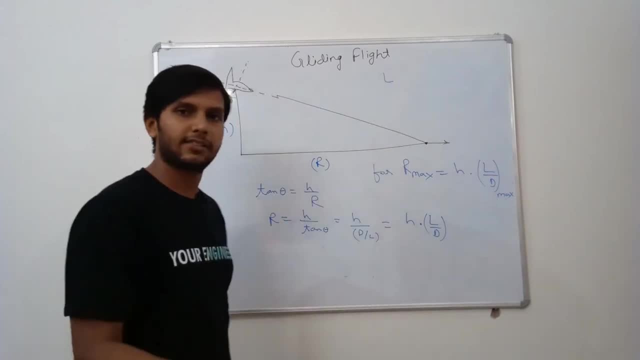 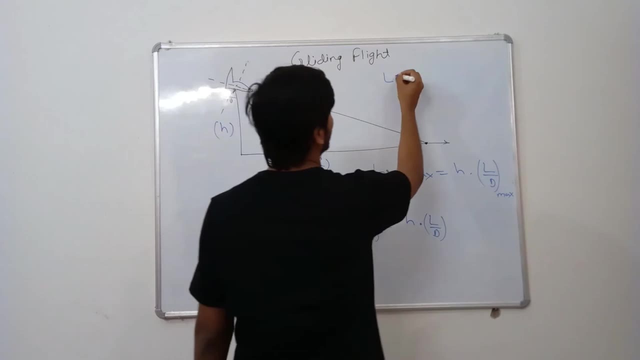 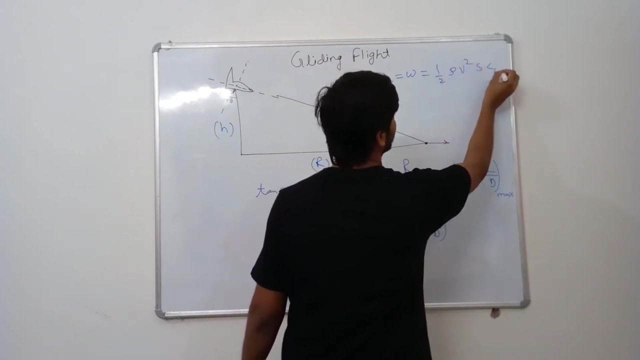 that our main formula, which is, when we take unaccelerated flight, steady or incompressible flight, and it is unaccelerated, in that case what will we take? We consider lift to be weight, Lift equal to weight which is half rho V square SC L. This formula comes out: We take the weight. 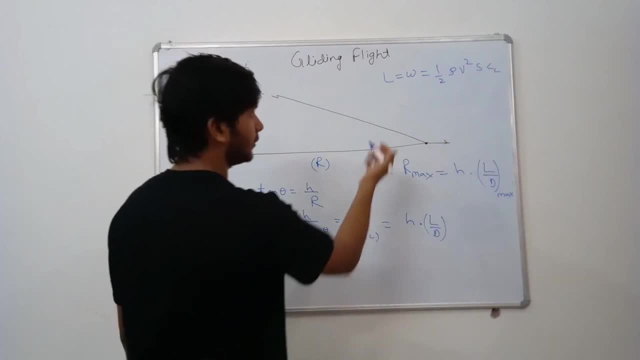 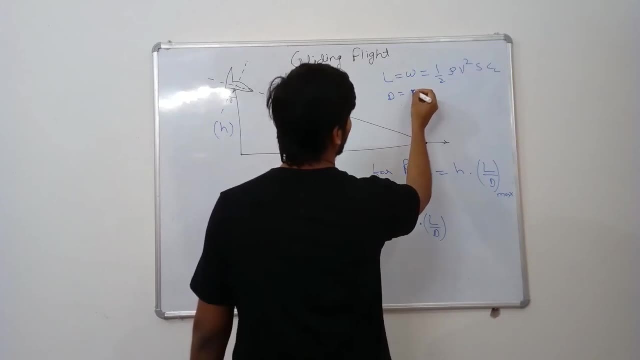 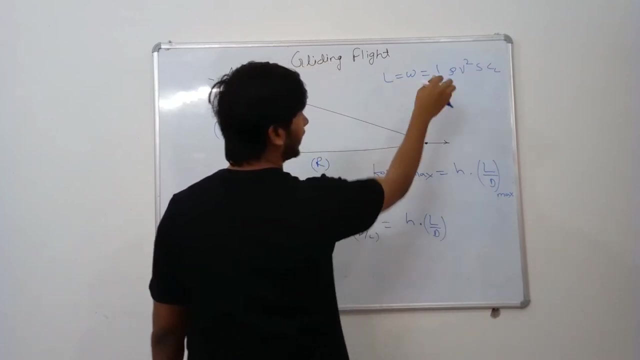 is given to the value of S over 0. same as drag, drag equal to w, drag equal to thrust. in that case it will be zero. but for now we will take lift equal to weight. so what formula do we have from here if we? 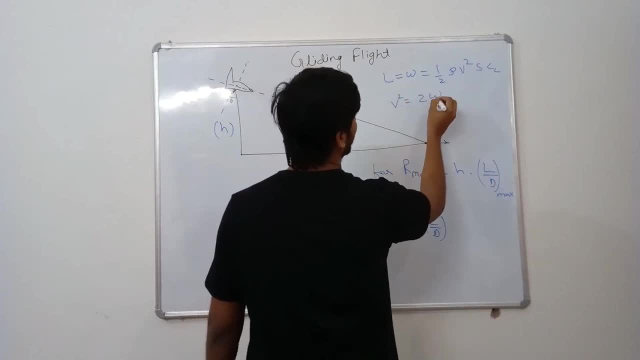 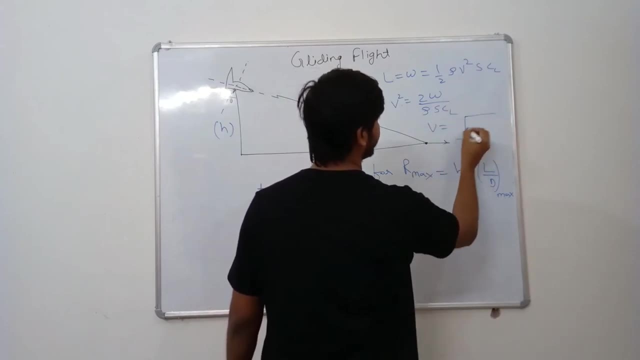 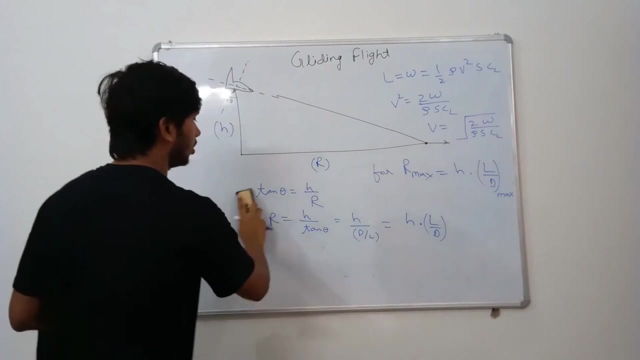 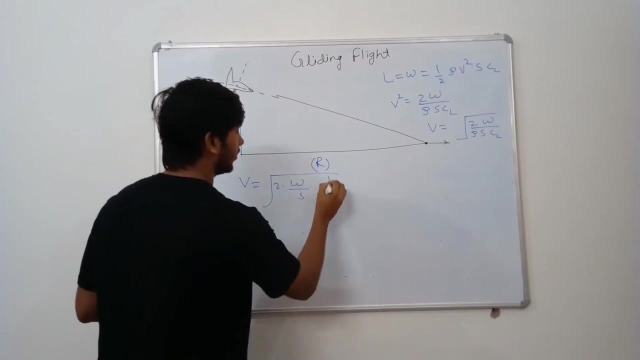 want to calculate velocity, then velocity formula will be v square equal to 2w by rho scl. so v formula will be square root of 2w by rho scl. we will see this better. so if I write it like this: v is equal to square root of 2 times w by s into 1 by rho cl. so 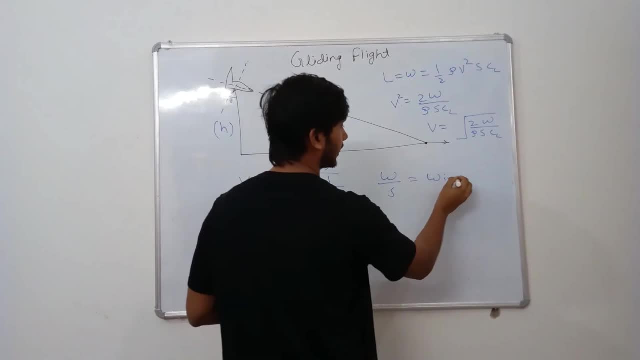 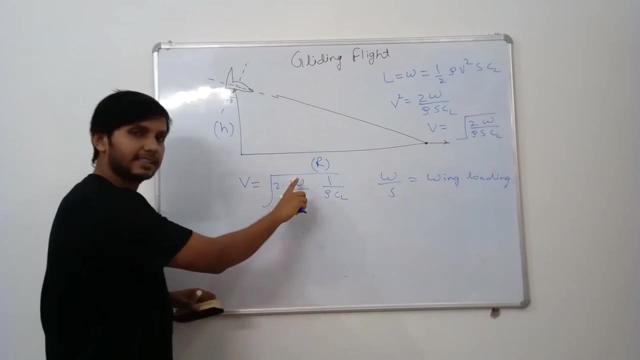 w by s is equal to square root of 2w by rho scl. So what we call it as wing loading. so wing loading is called w by s. now one thing you understand: if w by s is more, then velocity will be more. this is just a matter of saying.